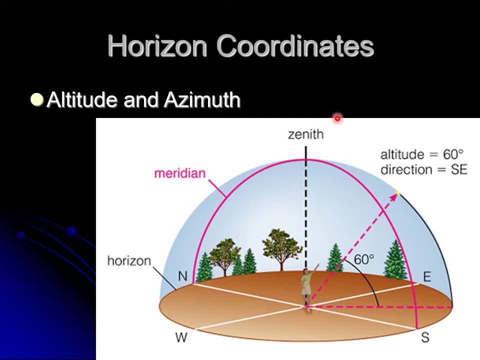 degrees, And so we would say 60 degrees. altitude is two-thirds of the way between the horizontal and straight up. We don't call it straight up, we call it zenith. Zenith is a term that means straight up. Things in the sky rise in the east and they set in the west. Well, they don't all go over straight. 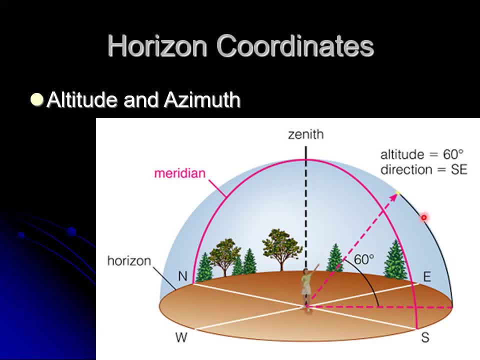 overhead. They sometimes cross, you know, someplace. They rise in the east and they cross here. So the highest they are in the sky is when they're in the midway between east and west. Well, that would be if you draw a line from north to south. If we draw a line from north to south and project. 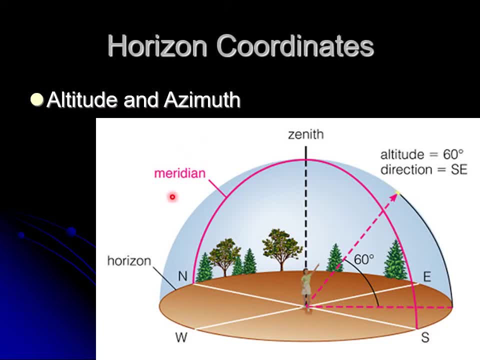 that onto the sky. we call that the meridian. So the meridian is this imaginary line that's going to cross the sky, running from north to south. So the highest anything is in the sky is when it's on the meridian. Well, we don't want to just say it's at a certain altitude, because over the course of the 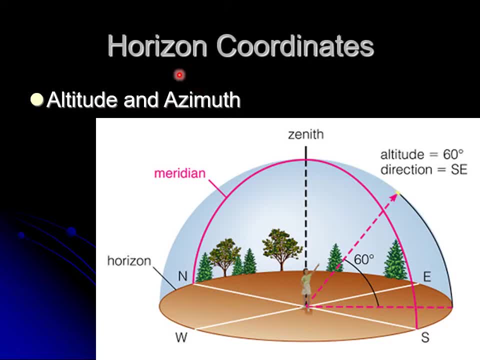 night things move. So we want to give what we also call the azimuth Altitude to how high above the horizon. Azimuth is what direction you're facing. So we start at north and we say north is zero azimuth. Measure an angle around this way. Well, that's right angle. So if you face east, you're facing right. 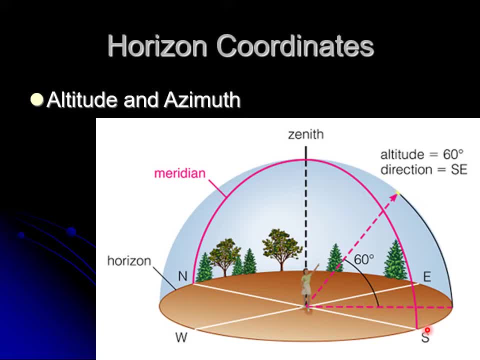 angles to north, And so that's 90 degrees. Okay, If something is due south, that's opposite north, So that is 180 degrees. West is 270 degrees. I know it's 90 degrees this way, but 270 degrees. 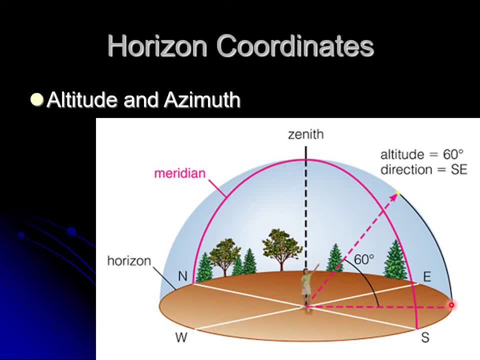 this way, we always measure to the east, And so if something is in the southeast, well, that's between 90 degrees and 180.. If you're exactly halfway between 90 degrees and 180, that'll be 135 degrees, And so we would say that. 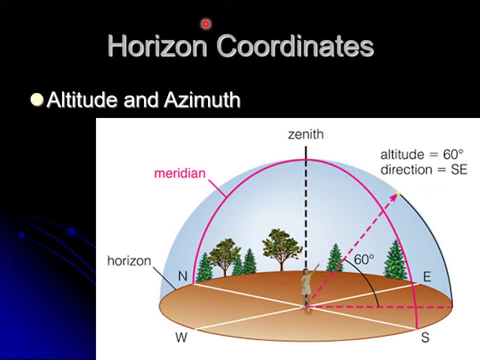 the azimuth is 135 degrees and the altitude is 60. That tells you, face southeast and look up 60 degrees, And that was where you look. So if I were to say, hey, I want you to go out and look at something. 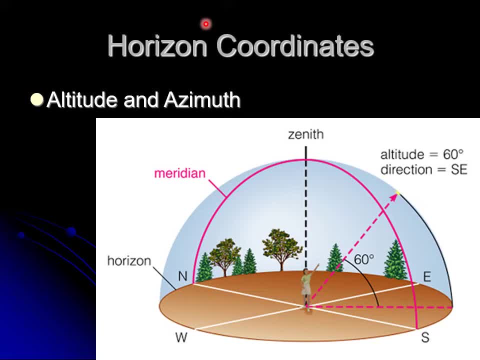 tonight I would tell you what direction to face and how high up to look to see it. That's the horizon coordinates. That sounds like a fantastic thing to do, except one problem: Earth is round. So different people on different parts of the earth look up in the sky and they see. 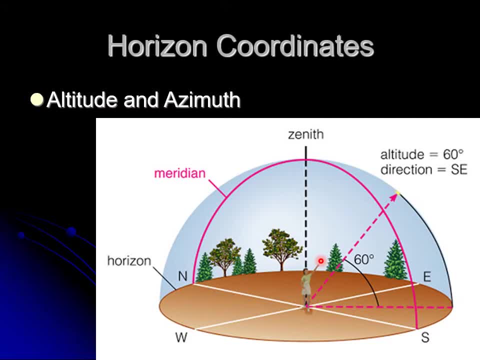 something different. The other thing is the earth's rotating, So that means that what's overhead now is not going to be overhead later. Things will rise in the east and setting them west, So they're always moving. So you would need to know exactly what time something is, a certain altitude and azimuth. 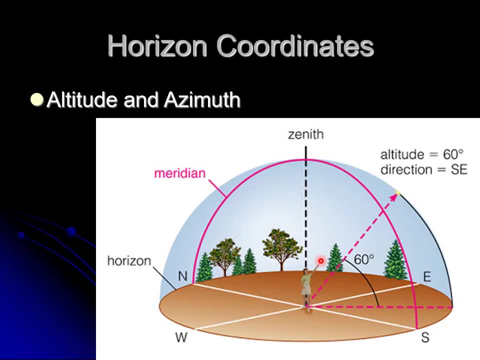 The other thing is, as earth goes around the sun, that shifts our entire perspective of the sky. So altitude and azimuth of an object is only good for a fraction here of a second or so at one particular moment in time from one particular location. So it's very much unique. 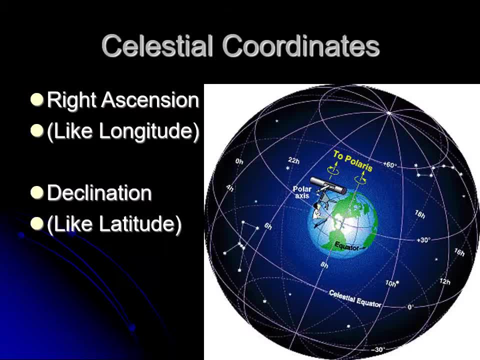 To the observer. We want to, So we do as we imagine the sky as being a big sphere here. OK, and again, you know, if you're at one location- the earth- you look up, you see certain stars at a different location. at the same time, you see different stars. 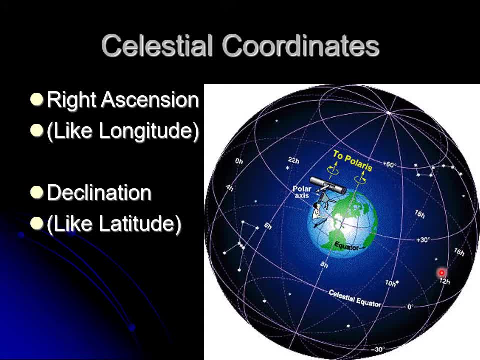 So you might have a star over here that someone in the Northern Hemisphere looks south to see. Some in the Southern hemisphere looks to the north to see Someone over here might look to the west, the east, to see it, and some of the other side of the world might look west to see it. 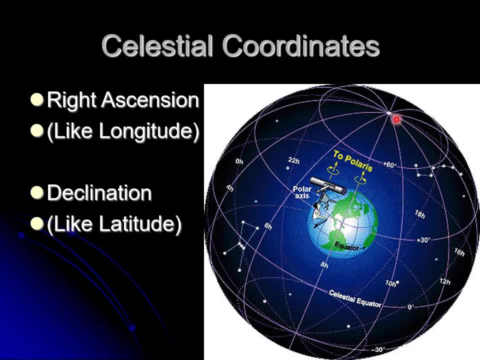 So it's going to be different for everybody. So we want to have coordinates on the sky. So when the sky is this big round thing, you know, we can imagine all the stars being on a sphere around the earth. Well, it's not really a sphere around the earth, but it makes it easy to map. 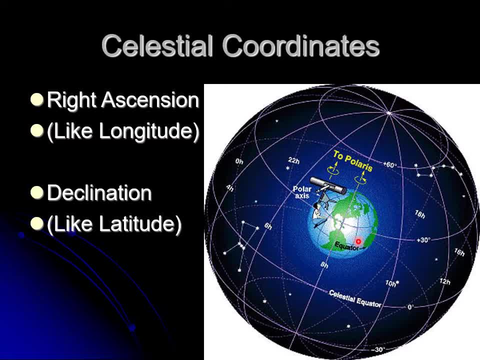 So we can draw what look like latitude and longitude lines across the entire sky. So we have longitude lines and then we have latitude lines. Now, like on earth, latitude is measured north and south of the equator, As the earth is sitting here spinning. 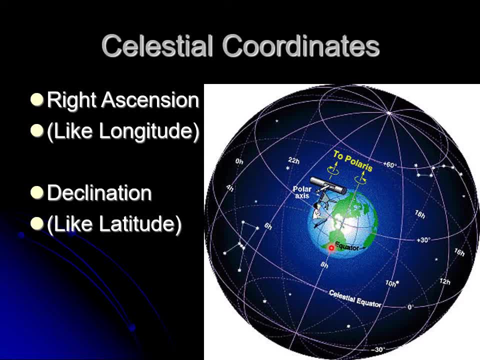 then the equator marks the midpoint between north and south pole And so everywhere on that equator you see as the earth rotates. you see stars right along there appear overhead If you're the north pole of the earth, because the earth's rotating. 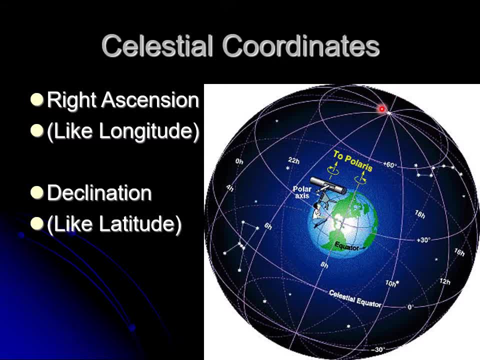 you see the same thing overhead all the time and the whole sky looks like it's going around that point. So it looks like the whole sky has a north pole and a south pole and an equator. So in fact we call that the north celestial pole, the south celestial pole and the celestial equator. 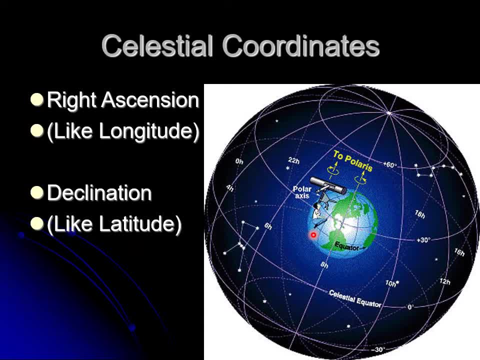 On earth. latitude is measured relative to the equator. The equator is considered zero. So where we live here in Fort Worth, Dallas area- okay, that's about 32 and a half, depending on where you are In Tarrant County. southern part of Tarrant County is close to 32 degrees. Northern part of Tarrant. 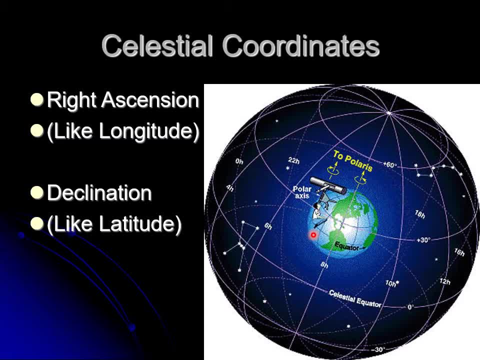 County is close to 33 degrees latitude, And so that's going to be north of the earth's equator. Now the interesting thing is, this is useful for navigation purposes, because if you're 33 degrees above the north of the earth's equator, you look up, you see something in the sky: 33 degrees. 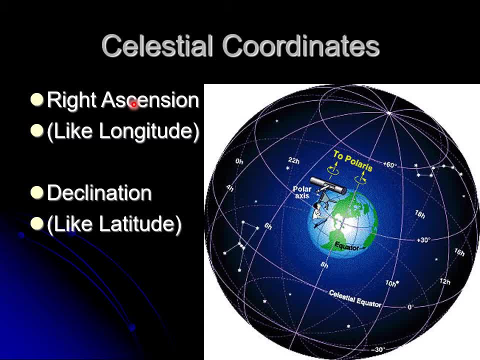 North of the celestial equator. So that's one reason that they do this is it helps you with navigation. If you have a map of the sky you can look up and see well, what declination is overhead and that would tell you what latitudes you are: Longitude, celestial longitude. Now on 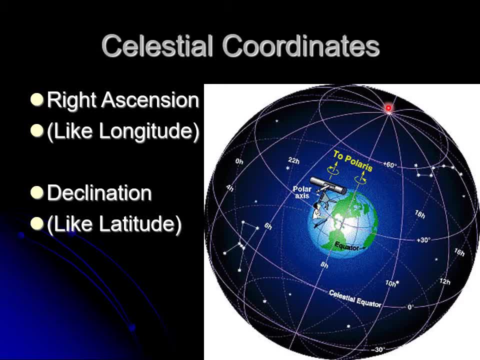 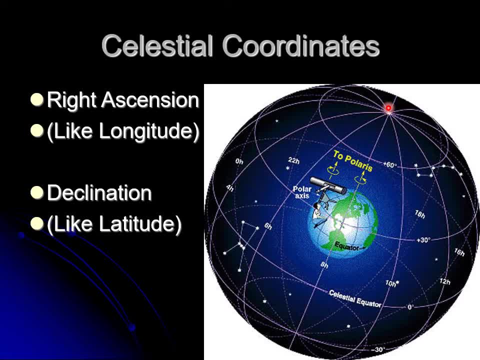 measure west of it. So in the sky, we want to have these lines that run from the north pole to the south pole and we want to measure. Okay, Now they decided, instead of calling it celestial latitude and celestial longitude, it's called declination. That's your latitude, And then 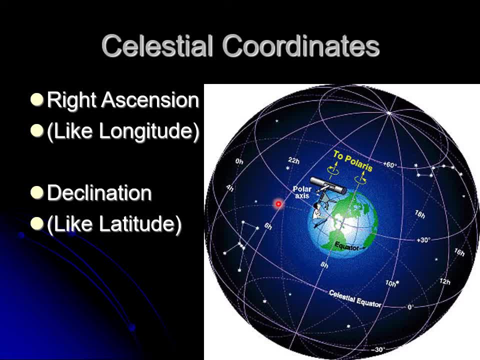 right ascension, that's your longitude. Now, the other thing that's different about the celestial longitude: the right ascension is, instead of measuring east and west, you know they realized, if you're standing out there looking the entire as earth rotates, the entire sky looks like it's. 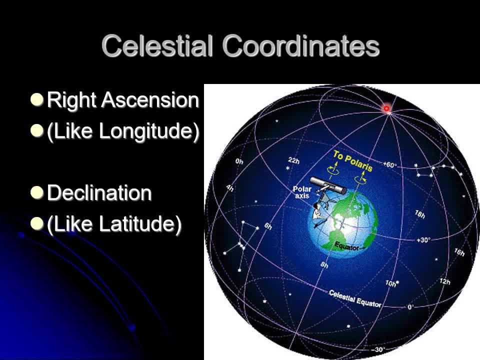 passing overhead. So if you wait 24 hours, yeah, I know the sun comes up, but there's still stuff up there. Everything goes in one direction. So what they decided to do was draw a line, call that zero and then just measure in one direction, to the east of that, And so it doesn't. 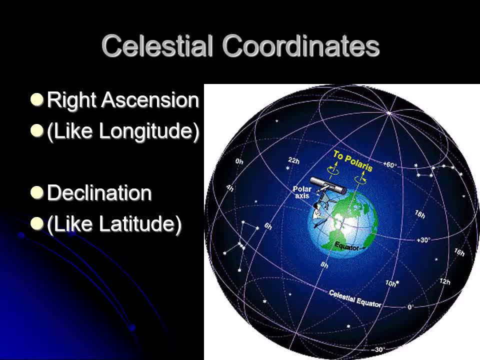 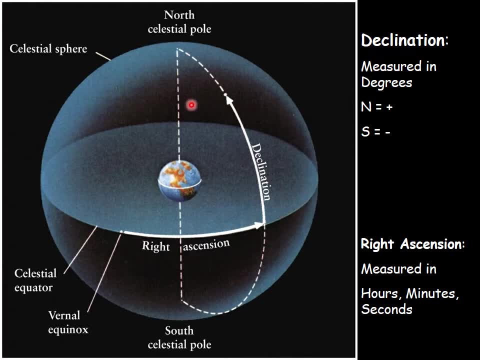 go east or west, it just starts and goes all the way around. Okay, So right. ascension has a starting point and it just measures in one direction all the way around. Declination measures north and south of the celestial equator. We don't call it north and south, we call it plus and minus. So if 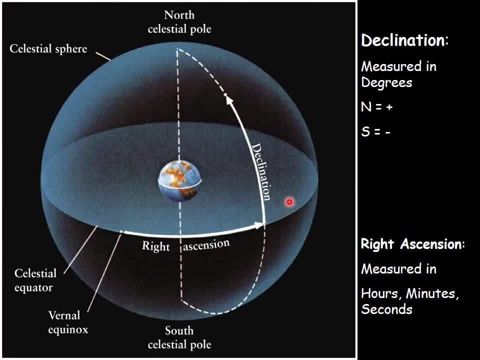 something is plus 45 degrees declination, that means it's 45 degrees north of the celestial equator. Now, right, ascension, pick a starting point, and we just measure in one direction. except we don't measure in degrees, we measure in hours, minutes and seconds, and so that would be. that's one thing that confuses students. 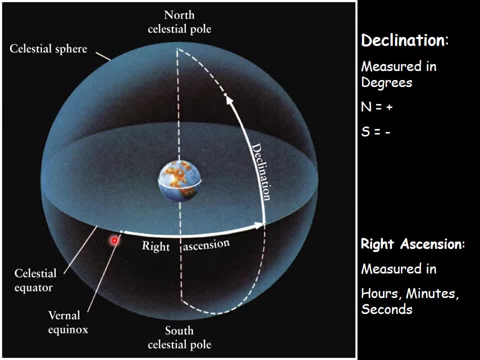 it's like you look up in the sky and if you look to the north you would see a star and the star might be like two degrees. it might be like 30 degrees to the north and you'd say that's 30 degrees to the north. but if it's 30 degrees to the east you don't say 30 degrees to the east. 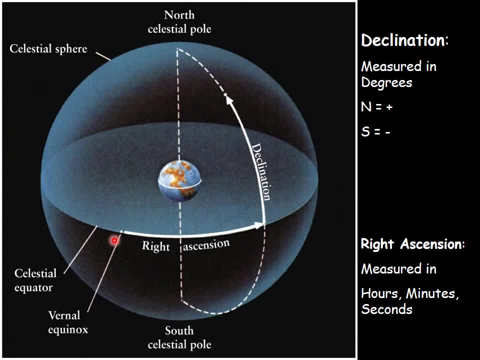 you say it's a difference of two hours. so why would you measure in hours, minutes and seconds? well, that's because earth is rotating. remember, i said you use this for not navigation purposes, but what happened is you would find a star and it's not directly overhead. uh, you would measure. 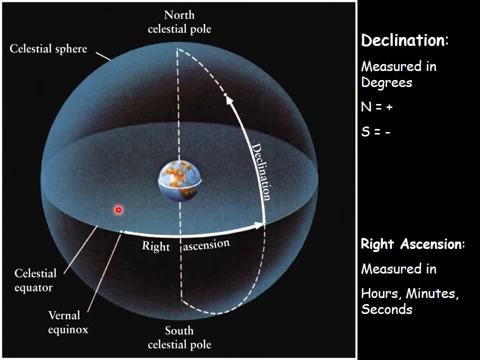 how you'd figure out how long it would take until it's overhead and if it's going to be in the future. that means that you happen to be a certain distance where of the prime meridian. if it's going to be in the other direction, you're going to be that far east. 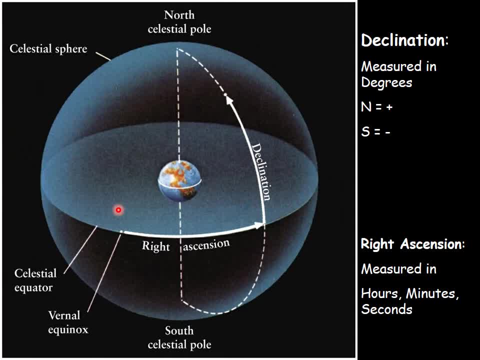 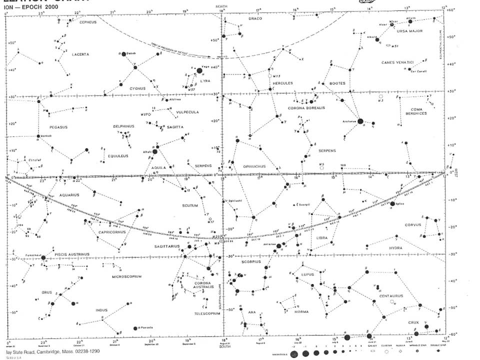 of the prime meridian, and so you would measure hours, minutes and seconds and then convert that to degrees, and so it was easier for astronomers- particularly the early ones that were using this for navigation purposes- only to measure in hours, minutes and seconds, and it's kind of a piece. 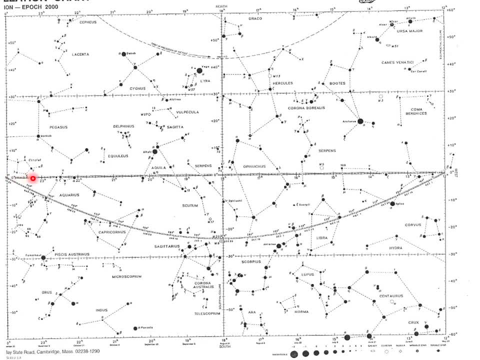 of a map of the sky, you know, that shows the celestial equator across the middle. okay, here's the declinations, the star and that. so we have a star that's right up here and that star has a declination of about 18 degrees. the right ascensions are marked over here. so this is zero hours. so that's zero hours. that's 23, 2 hours. 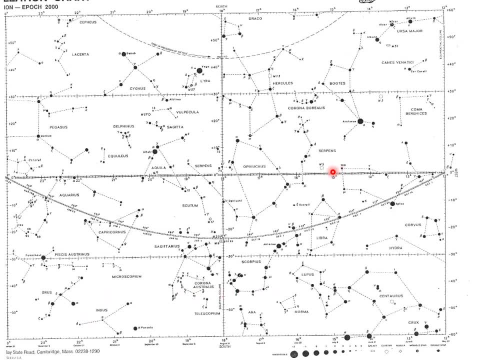 so the numbers are going bigger this way, and so what happens is right here, uh, this star, uh uh. if you look, uh, uh with the, the right ascension, this is for the star and that star is. the important thing is that you can measure it and that number is zero, because if you do, when you're right away, here is 22 numbers. now it's a Tierney number. 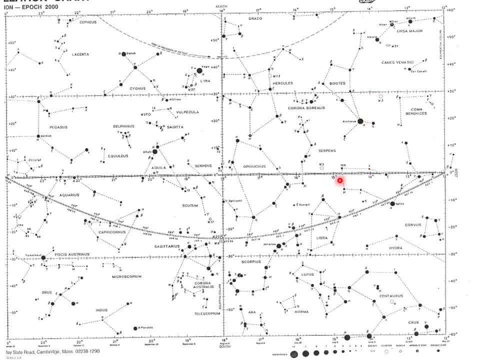 for the top of the scale. so 22 will go to zero in priority hours and 25 will go to ruining history of radioqueries. 14 hours right there, That's 15 hours. So that's about a quarter of the way. Well, we don't say. 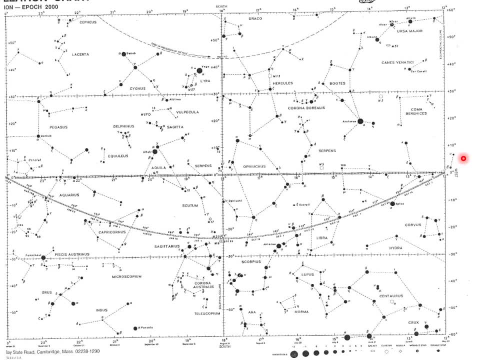 14 and a quarter. We say 14 hours and 15 minutes, And so that's how you would, that's how you would read that sort of thing. Okay, Does that make sense? Well, we were in class in person because 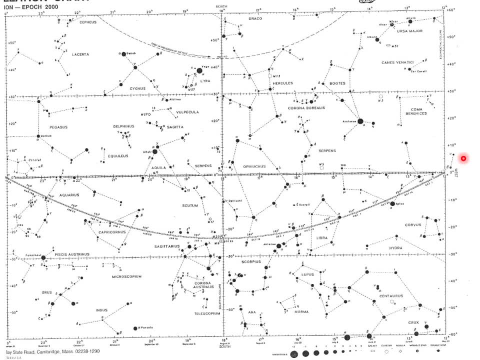 then you could say yes or no, and I could give more examples. But one of the first labs that you're going to be doing is celestial coordinates, and it gives you a little more practice. Now notice that on this map and on the star maps you're going to use, west is on the right side. 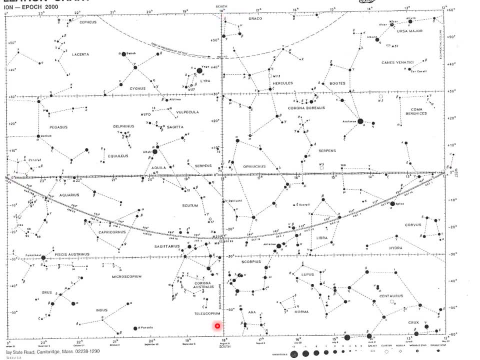 and east is on the left side, North's at the top, south's at the bottom, but east and west are backwards. Well, why is that the case? Well, because this is meant to be held up over your head, looking out. Most maps that you learn to read are looking down onto the 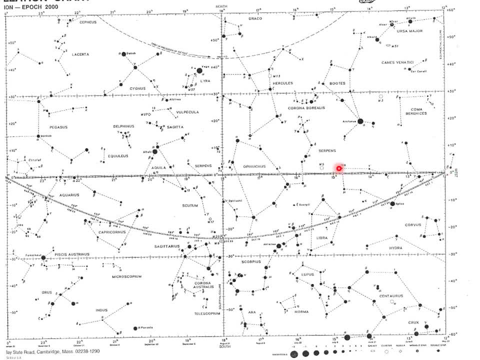 earth, And so that's what we're going to be doing, And so that's what we're going to be doing. This is on the earth looking up and out, So east and west are backwards, So this way is west, that way is east, this way is north and that way is south, And so that'll help you.